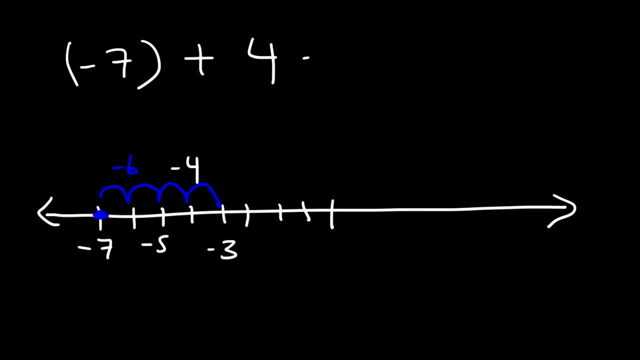 negative 5, negative 4, negative 3.. So negative 7 plus 4 is negative 3.. And that's a simple way in which you can add two numbers. Now what about adding two large numbers Without the use of a calculator? Let's say 175 and 86.. It's helpful if you. 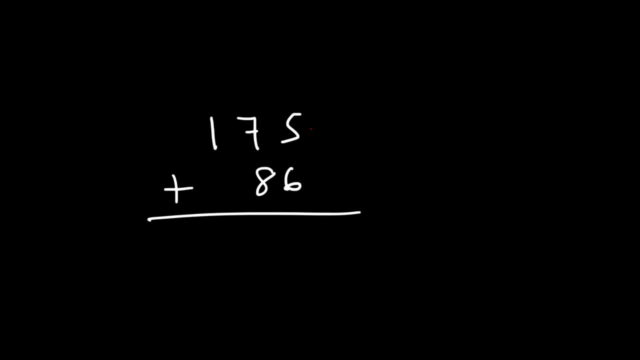 align it this way And what you want to do is add the numbers in each column. So first we want to add 5 plus 6.. 5 plus 6 is 11.. So we're going to write the second number in 11 and the first number we're going to carry it over. Next we're 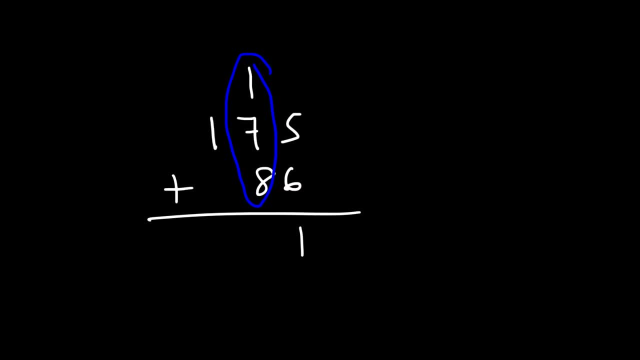 going to add 1 plus 7 plus 8.. 1 plus 7 is 8.. 8 plus 8 is 16.. So what we're going to do is write the second number, carry over the first one, And now we just have 1 plus 1, which is 2.. So the 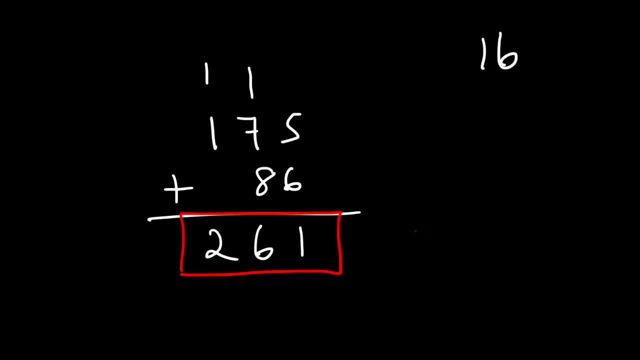 answer is 261.. And so that's another way in which you could perform simple addition. The second skill that you need to know is subtraction. So let's say, if we wish to subtract 9 by 3.. What's the answer? Well, if you're dealing with small numbers, you could use a. 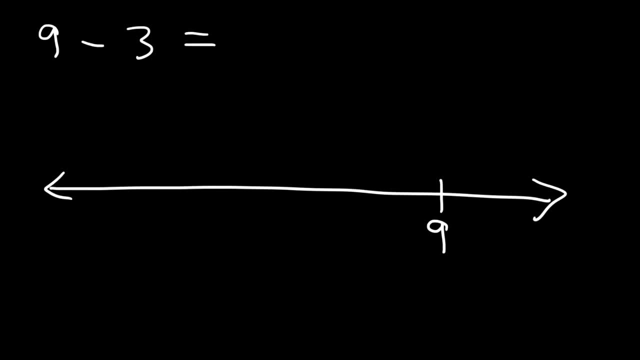 number line. So let's say 9 is right there. Now, if you're adding, you want to travel to the right of the number line, But if you're subtracting travel to the left of the number line. So if we wish to subtract 9 by 3, we need to. 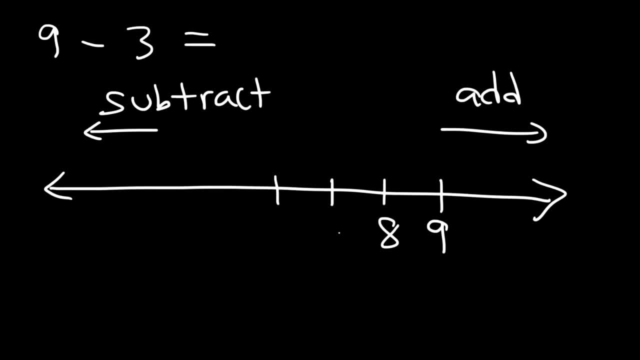 travel 3 units to the left. So this is going to be 8,, 7, and 6.. So 9 minus 3 is equal to 6.. Now let's try another example. Let's say if we have a negative 6 minus 5. Feel: 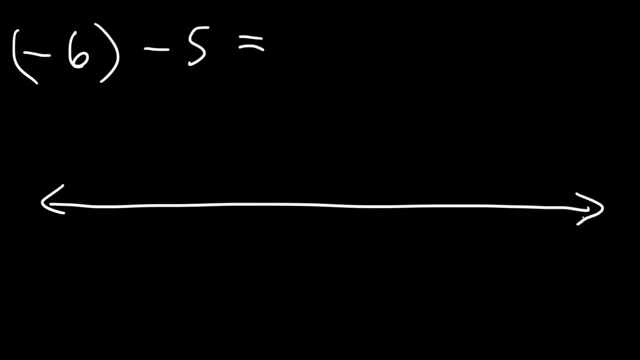 free to pause the video and try that one. So let's say this is 0 and this is negative 6, which is to the left of the 0. So we subtract a negative 6 by 5, which means we need to travel 5 units to. 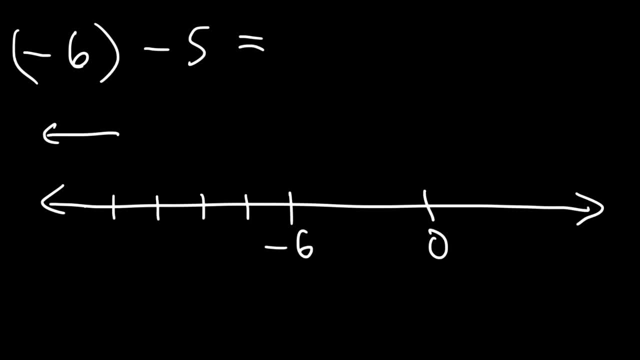 the left: 1,, 2,, 3,, 4, 5.. So this is negative 7, negative 8, negative 9, negative 10, negative 11.. So negative 6 minus 5 is negative 11.. Now what about this example? What's negative 4 minus negative 3?? 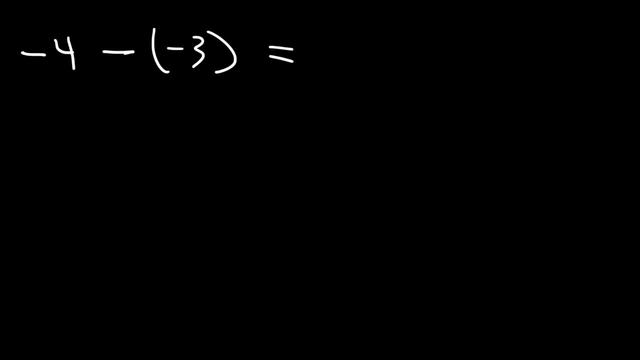 Before you use a number line, you need to simplify this expression. It's important to know that a negative times a negative is equal to a positive number, So negative 4 minus negative. 3 is equal to a positive number, So negative 4 minus negative. 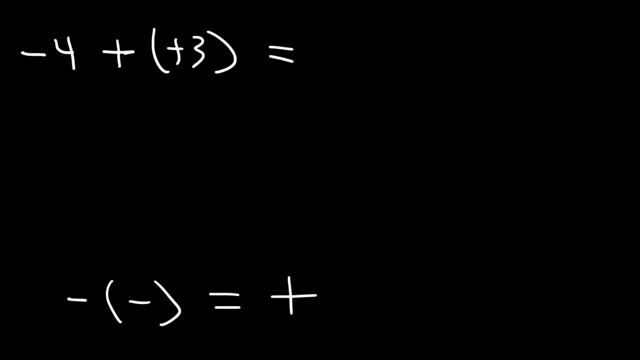 3 is really the same as negative 4 plus 3.. So now let's use the number line. So let's start with negative 4.. So we're adding 3 to negative 4, which means that we need to travel to the right side. So we got to travel 3 units to the right. 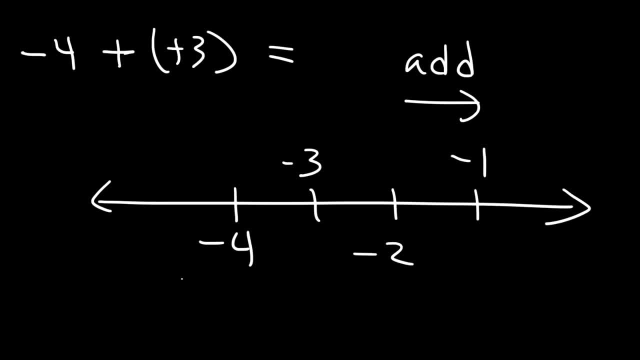 This is going to be negative 3, negative 2, negative 1.. So negative 4 plus 3 is minus 1.. Now let's work on some examples. We we're using negative 3 together and we're gonna divide this inгрings. 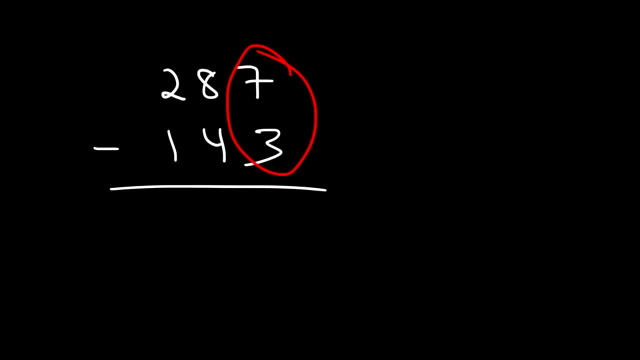 into two. That's negative 3 minus negative 3.. Pine number minus 2 is 5 and negative 3 is negative 6, as negative two. So the answer is negative 4 minus negative, 4 minus negative 3.. Now here's. 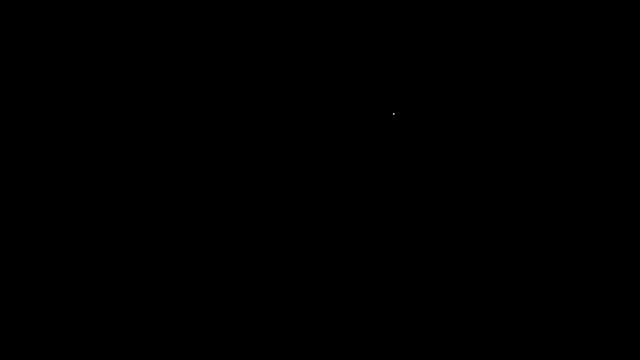 another example of subtracting large numbers. So what is 287 minus 143?? This one is going to be a little bit harder than the last one, So go ahead and subtract 342 by 176.. So let's start with the first column on the right. 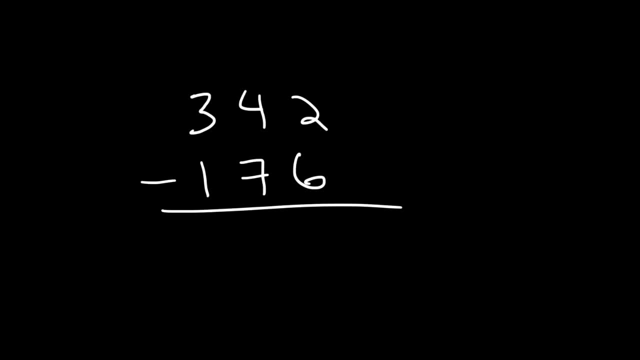 What is 2 minus 6?? Now, 2 minus 6 is a negative number. So what you need to do in this situation is you need to borrow a 1 from the 4. So the 4 becomes a 3, and the 2 turns into a 12.. 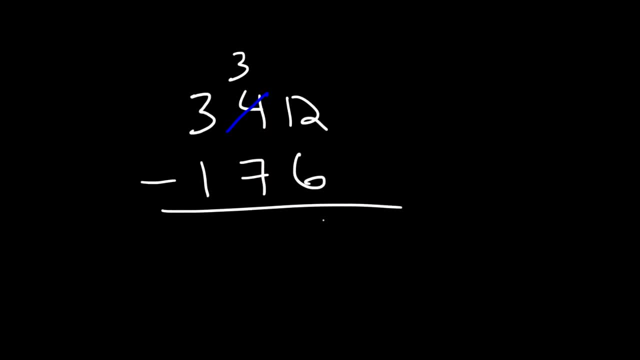 So now what you're doing is 12 minus 6.. 12 minus 6 is 6.. Now let's move to the second column. We can't subtract 3 by 7, because it's going to give us a negative number. 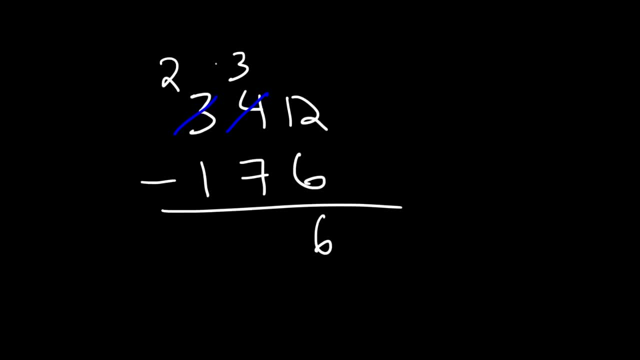 So what we need to do is borrow a 1.. The 3 becomes a 2, and we're going to transfer the 1 to the 3 in the middle, So this 3 becomes 13.. 13 minus 7 equals 1.. 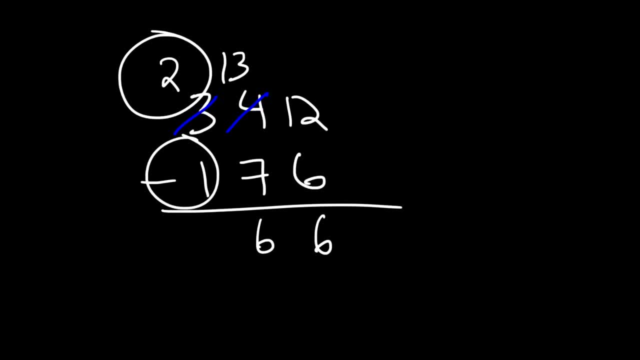 It's 6.. And lastly, we have 2 minus 1, which is 1.. So the answer, 342 minus 176, is equal to 166.. And you can confirm this answer with a calculator. Now let's talk about the third math skill that you need to know. 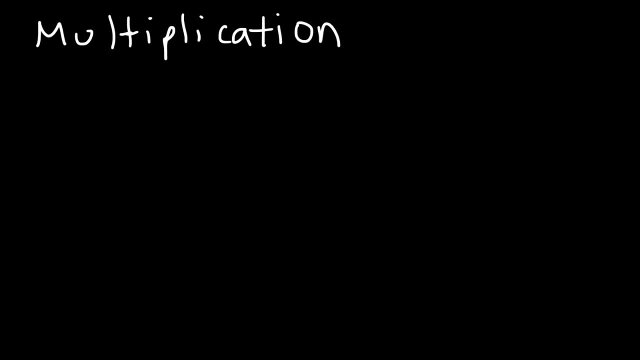 And this one is called multiplication. Now you might be wondering: what is multiplication? Multiplication is basically repeat, addition. Let me illustrate it. Let's use a simple example: 3 times 2.. Now you know, 3 times 2 is 6, but let's think about what this expression really means. 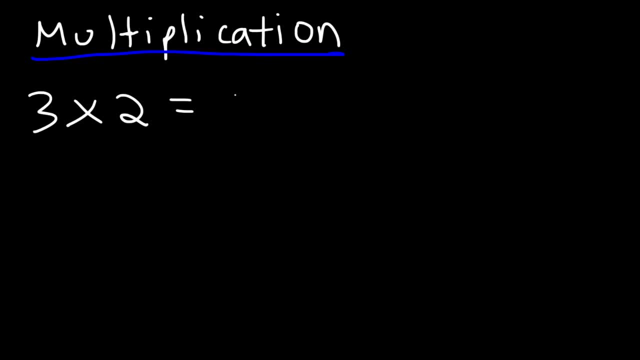 It can mean one of two things: 3 times 2 is equivalent to add in 3 two times, or add in 2 three times 3 times 2 is equivalent to add in 2 three times. 3 times 2 is equivalent to add in 2 three times. 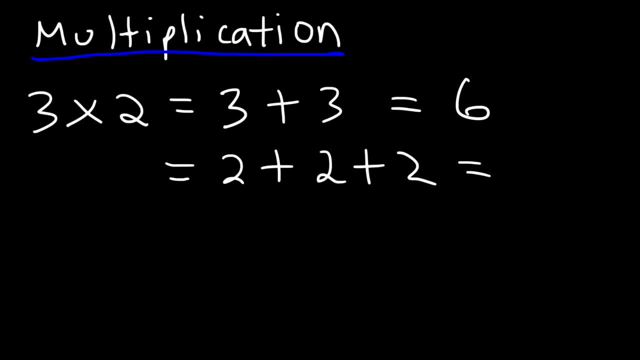 3 times 2 is equivalent to add in 2. three times 3 plus 3 is 6.. 3 plus 3 is 6.. 2 plus 2 is 4.. 2 plus 2 is 4.. 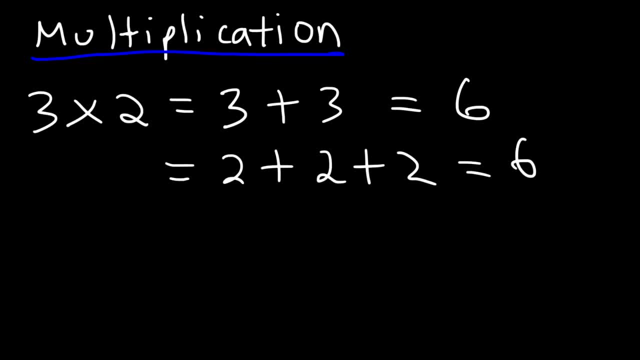 And 4 plus 2 is 6.. So you get the same answer. Now let's use another example to illustrate this: 5 times 4.. So 5 times 4 is equal to add in 5 four times. or you can add 4 five times. 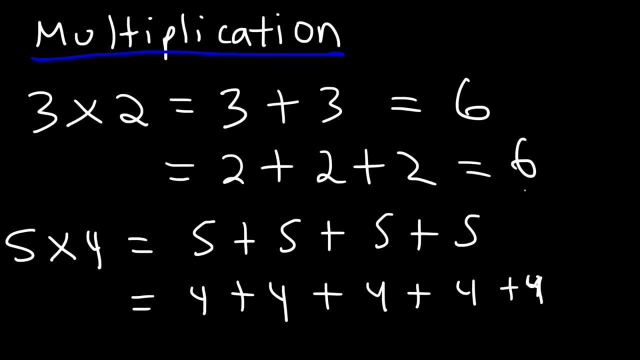 So thus you can see why multiplication is really repeat addition. Now let's look at multiplication Now: 5 plus 5 is 10, and so this is another 10,. 10 plus 10 is 20.. Here we have 4 plus 4, which is 8, and then 8 plus 4 is 12,. 12 plus 4 is 16,, 16 plus 4. 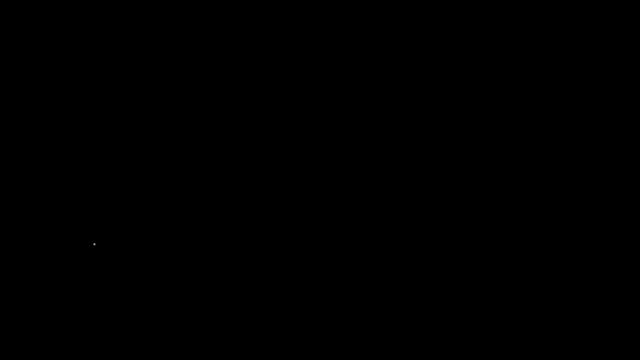 is 20.. Now, let's say, if we wish to multiply 13 by 20,, what would you do? There's different ways in which you can do this. Now, some people are not good with math, but when it comes to money, math makes sense. 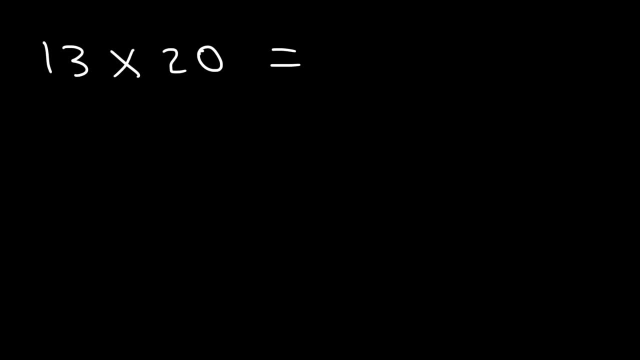 Imagine if you have 13 $20 bills. How much money do you have? So let's draw that, So let's say this represents a 20.. Here is another 20, and you know that 5 20s add up to 100. 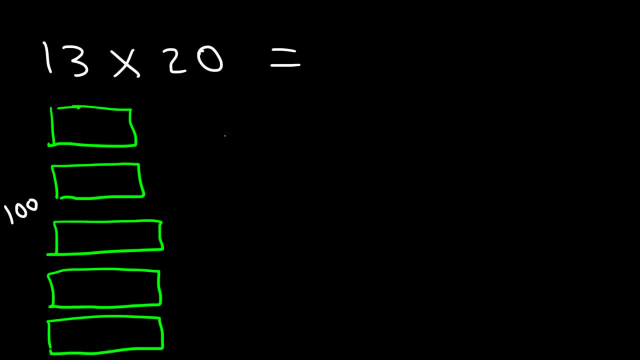 So right now that's $100.. And here's another 5 20s, Here's another 20.. Here's another 20.. So that's another $100.. And then here we have 3 20s, So we have a total of 13 20s. 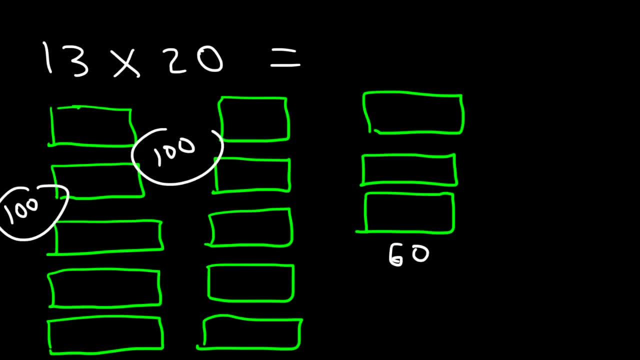 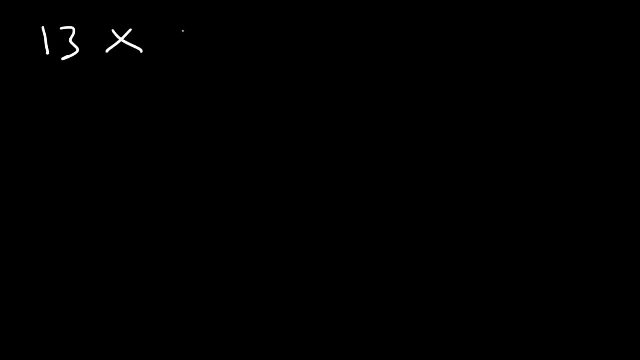 3, 20s is 60. So 100 plus 100 plus 60 is 260. And so, if you can relate math to money, multiplication and addition becomes very easy because you can visualize it. Now there's another way in which we can get the same answer. 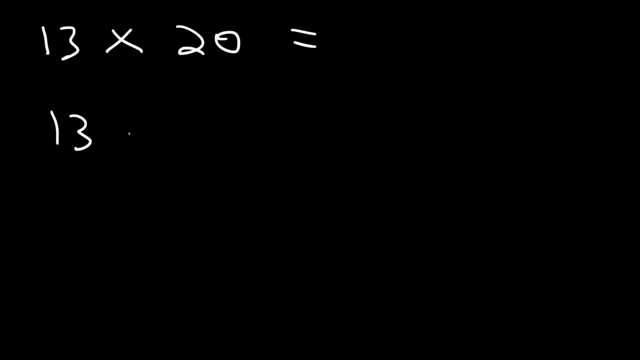 What is 13 times 2?? Now, 13 times 2 is basically adding 13 two times. So if we align the two numbers, we can see that 3 plus 3 is 6, and then 1 plus 1 is 2.. 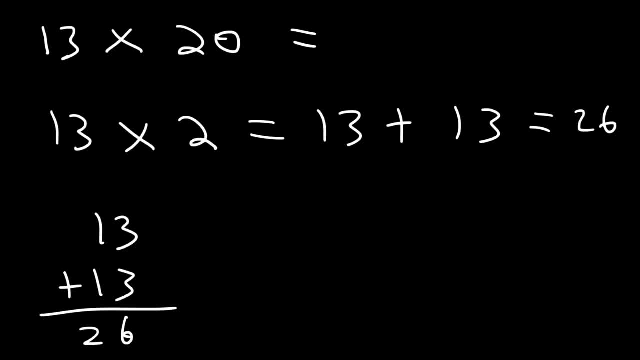 So 13 plus 13 is 26.. Now if 13 times 2 is 26,, what is 13 times 20?? All you need to do is add the 0.. So 13 times 20 is 26 with 0, or basically 260.. 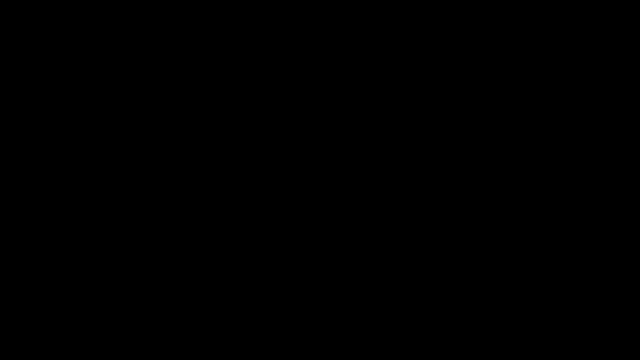 So there's many ways in which you can simplify multiplication. Now let's try another example. What does this expression mean? If you see two numbers next to each other without a plus or minus sign between them, it means multiplication. So we're multiplying 7 by 26.. 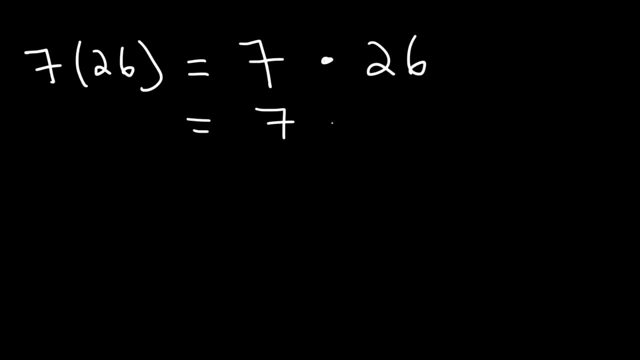 So what is 7 times 26?? One way in which you can get the answer is you can rewrite 26 as 20 plus 6, and then you could use the distributive property Seven times 20.. Well, what is 7 times 2?? 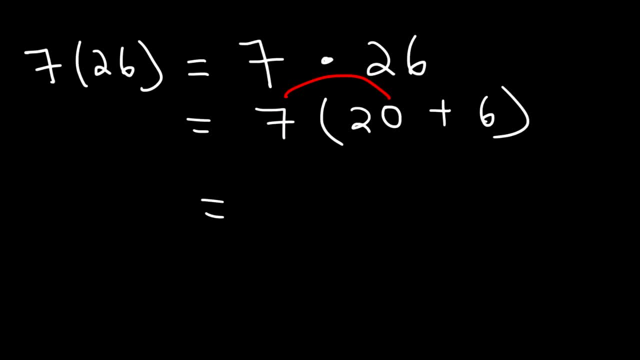 If you add 7 and 7, you get 14.. So if 7 times 2 is 14,, what is 7 times 20?? All we need to do is add the 0.. 7 times 20 is 140.. 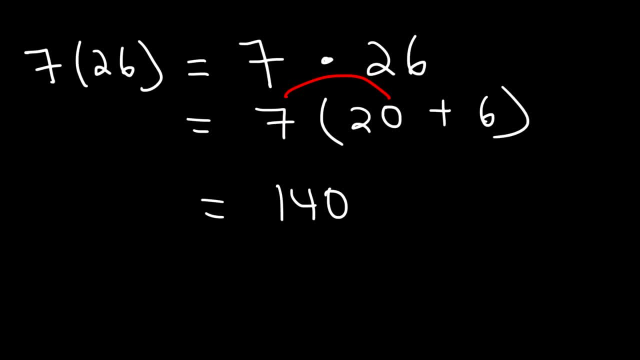 If you have seven $20 bills, you have $140.. Next, we have 7 times 6, which I hope you know. your multiplication tables: Seven times 6 is 42. And so 140 plus 42 is 182.. Thus, this is the answer. 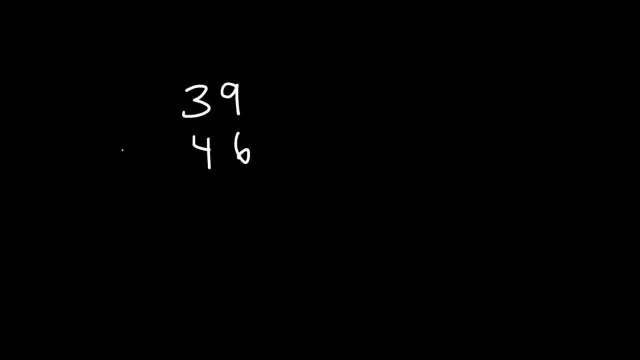 Now let's try some harder examples. What is 39 times 42?? What is 49 times 46?? What do we need to do here? The first thing you need to do is multiply 9 by 6.. Nine times 6 is 54.. 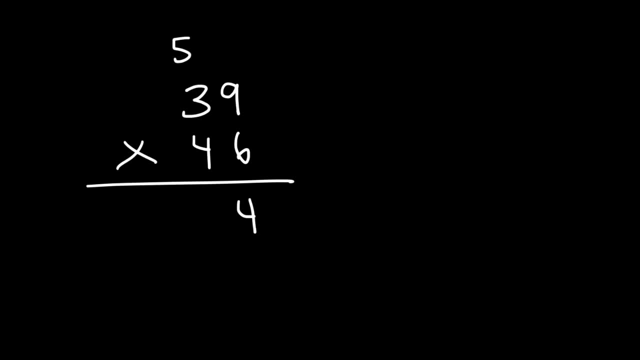 So we're going to write down a second number, but carry over the first number. Next, we have 3 times 6,, which is 18, plus 5.. And 18 plus 5 is 23.. Now what you need to do is write a 0.. 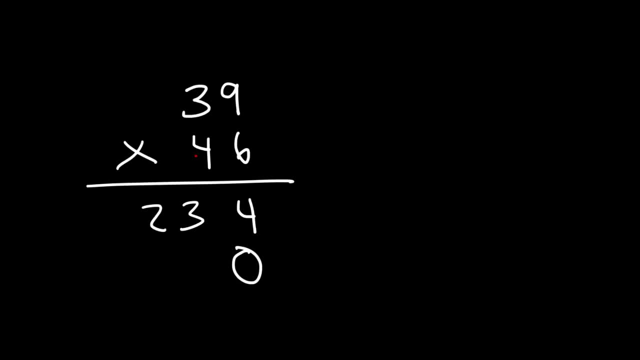 And then we're going to multiply 4 by 9.. Four times 9 is 36.. So we're going to write the 6 and carry over the 3.. Next we have 4 times 3,, which is 12, plus 3.. 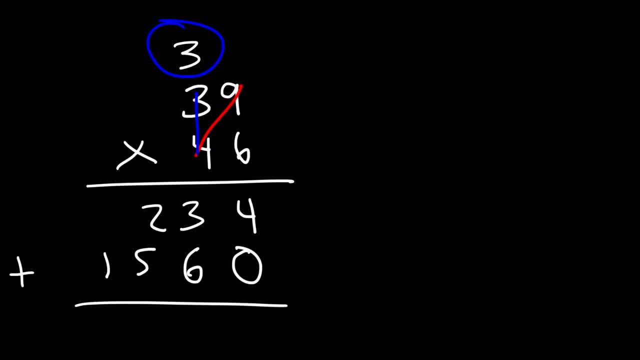 So that's 15.. At this point, what you need to do is add. So 4 plus 0 is 4.. 3 plus 6 is 9.. 2 plus 5 is 7. And we can bring down the 1.. 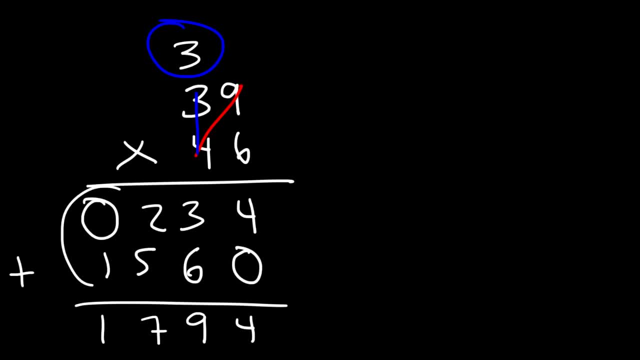 Or you can treat this as if it's a 0, and you can say: 0 plus 1 is 1.. Either case, the answer is 1794.. Now let's try another example. Let's multiply 326 by 37.. 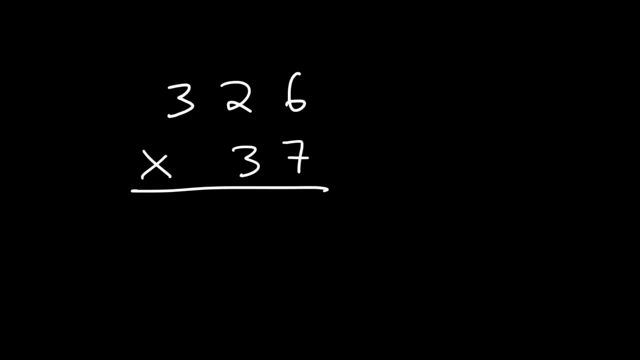 Feel free to pause the video if you want to work out this example. So let's begin by multiplying 6 by 7.. 6 times 7 is 42. So we're going to write down the second number and move the first number to the top. 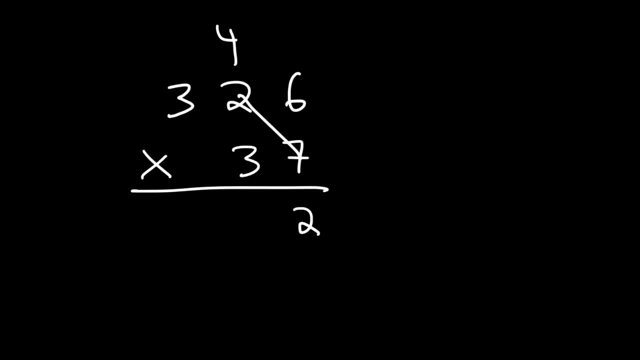 Two times 7 is 14, plus 4,, that's 18.. Now we're going to write down the 8,, carry over the 1.. Three times 7 is 21, plus 1, that's 22.. 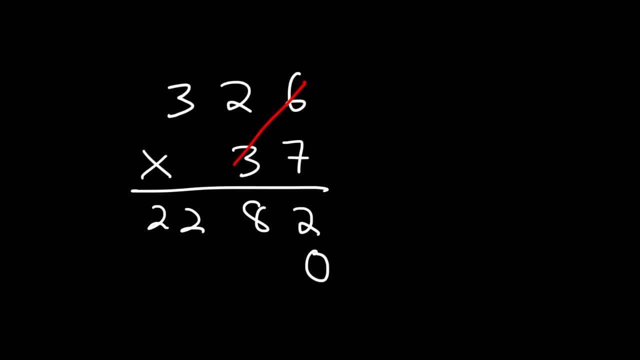 Now let's add a 0. And then we're going to multiply 3 times 6,, which is 18.. So we're going to write the 8, carry over the 1. It's going to be 3 times 2,, which is 6, plus 1,, that's 7.. 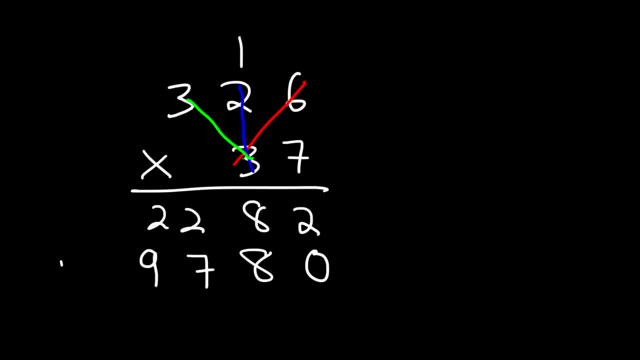 And then it's going to be 3 times 3,, which is 9.. So now let's add: Two plus 0 is 2.. Eight plus 8 is 16.. Write the 6, carry over the 1.. 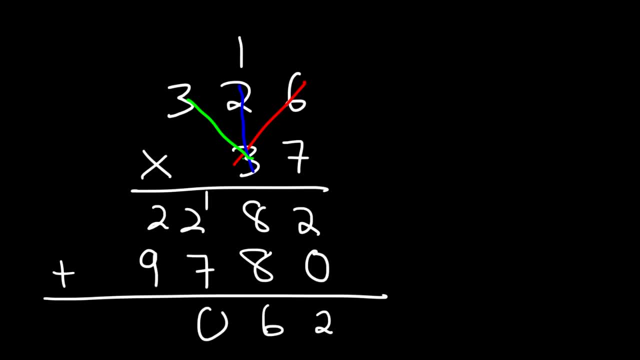 One plus 2 is 3.. Three plus 7 is 10.. Write the 0,. carry over the 1.. One plus 2 is 3.. Three plus 9 is 12.. So the final answer is 12,062.. 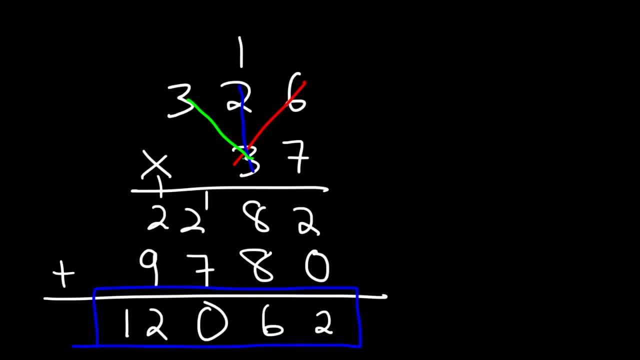 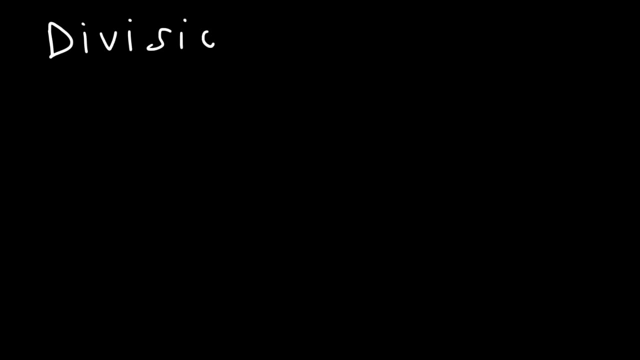 That's the answer, Thank you. So now you know how to multiply two numbers And you understand what multiplication really means, And it's basically repeat addition. Now let's move on to our next math skill, which is division. So what is division? 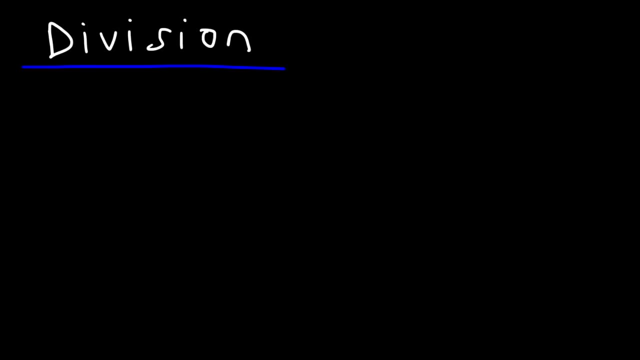 Division is the reverse process of multiplication. Allow me to illustrate. We said that 5 times 4 is 1.. 5 times 4 is 20.. Well, 20 divided by 4 is 5.. We could also say that 20 divided by 5 is 4.. 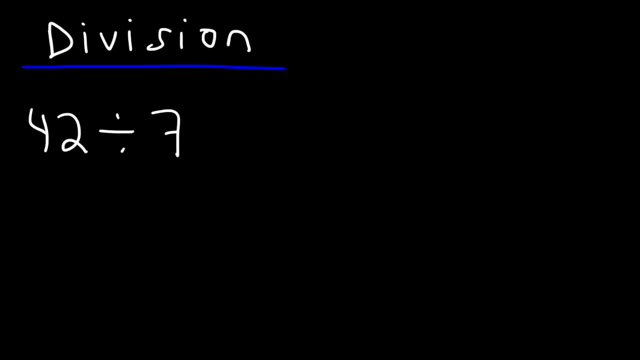 So let's say, if I wish to divide 42 by 7. I can also ask myself this question 7 times: what number is 42?? Now, using the multiplication, you can also ask yourself this question: What number is 42?? 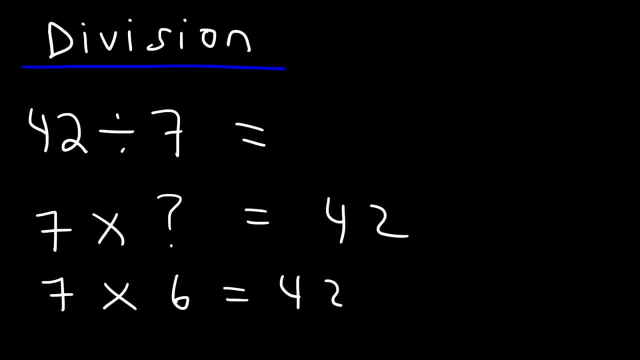 multiplication tables. I know that 7 times 6 is 42. therefore, 42 divided by 7 has to be the missing number, 6, and so that's the basic idea behind division. but now let's say if you have a large problem or a problem with a large number. 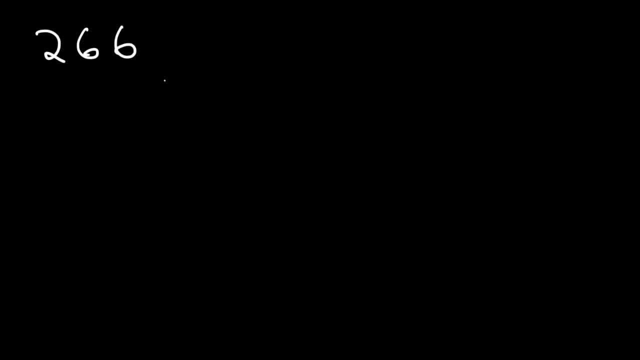 rather, let's say, if we wish to divide 266 by 7. by the way, if you see a fraction and you wish to find its value, you could find the decimal value of a fraction by using division. so this is the same as 266 divided by 7. now to 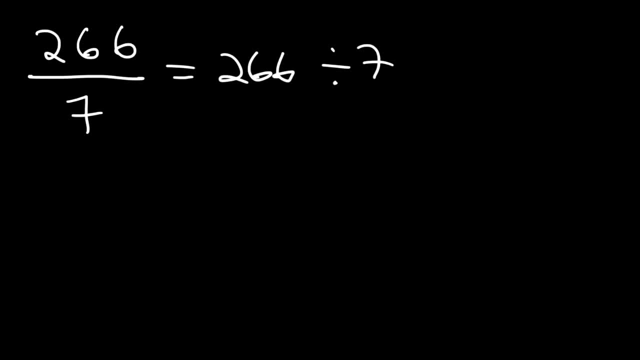 perform division of this sort, it's good to use something known as long division. so let's focus on the first two numbers, because seven doesn't go into two, because seven is greater than 2. 7 can go into 26 because 26 is greater than 7. 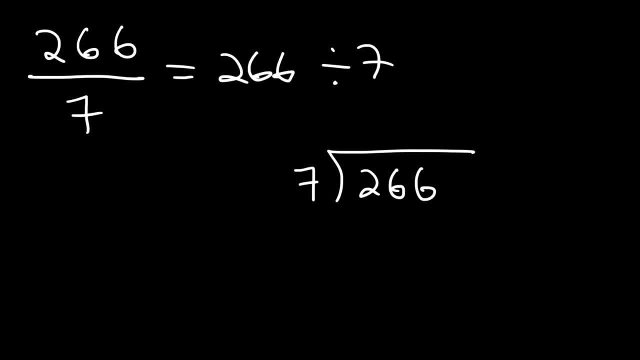 how many times can 7 go into 26? let's make a list. we have 7. 7 plus 7 is 14, 14 plus 7 is 21, 21 plus 7 is 28, and so forth. so this is one, two, three, four, five. 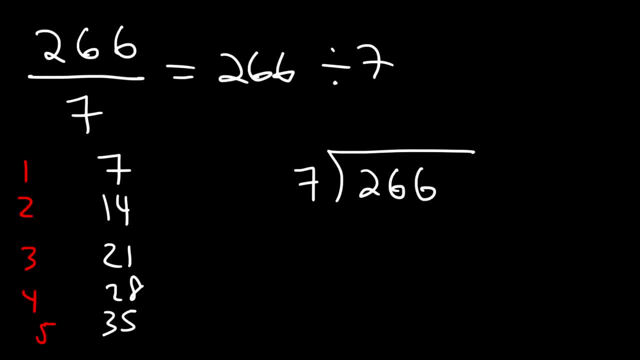 now you might be wondering: what are these numbers? why am i writing these numbers? well, seven times two is 14, 7 times 3 is 21 and 7 times 4 is 28. this is the process that I use when doing long division especially. 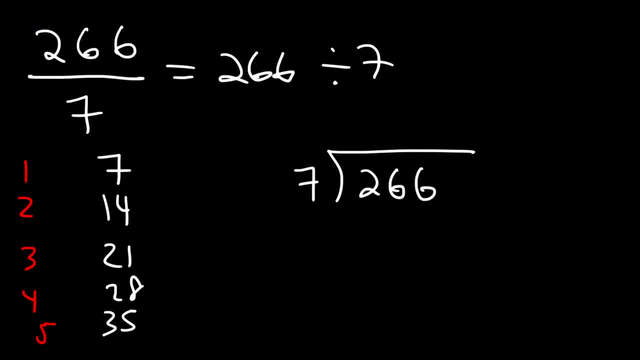 with large numbers. so this tells me that 7 can go into 2, 6, 3 times because 21 is less than 26. 7 doesn't go into 26 four times because 7 times 4 is 28 and 28 is larger than 26.. 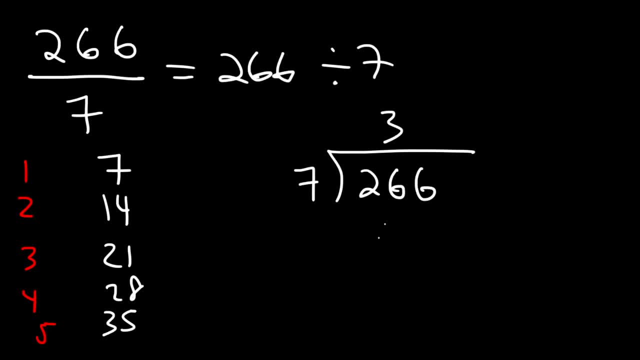 So what we need to do is put a 3 on top 7 times 3 is 21.. Next we'll need to subtract: 26 minus 21 is 5, and then we need to carry over the 6.. Now, how many? 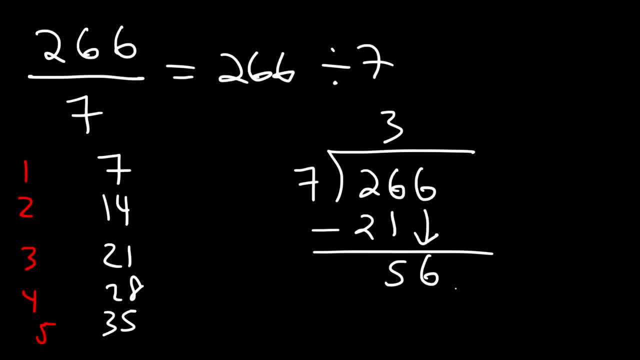 times does 7 go into 56?? 7 times 8 is exactly 56, and so now we have a remainder of 0.. Our answer is on top. So 266 divided by 7 is 38, or we could say that 38 times 7 is 266.. Now let's work on another example. What is two thousand? 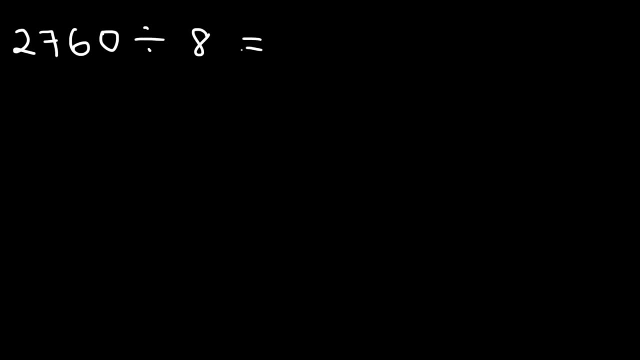 seven hundred and six sixty divided by 8?? Go ahead and try that. So let's write out the sums of 8.. So 8 plus 8 is 16.. 16 plus 8 is 24, and then we have 32,, 40,, 48,, 56,, 64,, 72, and 80. You really don't need to write out the numbers. You just need to write out the numbers. You really don't need to write out the numbers. You just need to write out the numbers. You really don't need to write out the numbers. 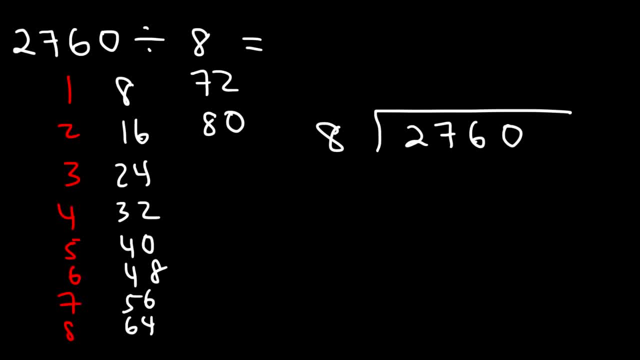 You really don't need to write out the numbers. You don't need to go past 10.. Once you get up to 10, you can stop. So how many times this 8 goes into 27.. 8 goes into 27 three times because 32 exceeds 27.. 24 is the highest multiple of 8, just under 27.. 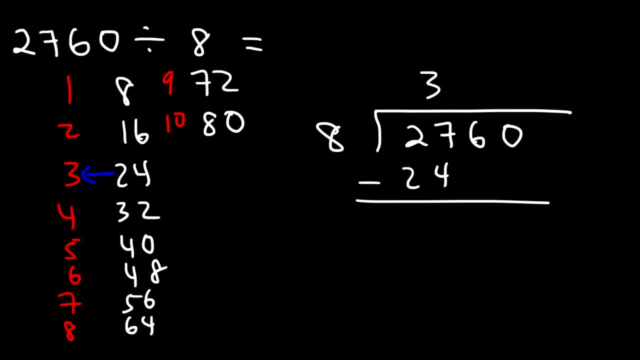 So 8 times 3 is 24, and on 27 minus 24 it will be 3.. Now let's over down to 6.. So how many times does 8 go into 36?? What's the highest multiple of 8? just under 36?. 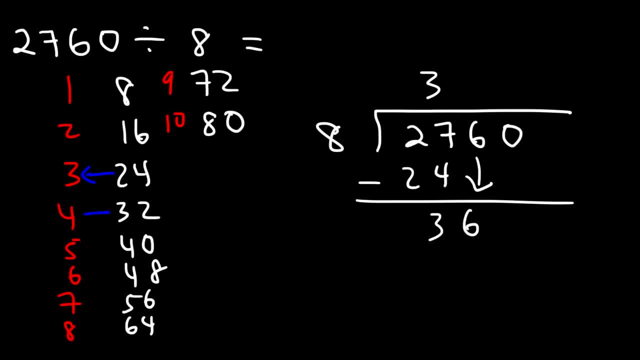 The highest would be 32.. So we could say that 8 goes into 36 4 times. 8 times 4 is 32.. 36 minus 32 is 4.. Now let's bring down a 0, and we can see that 8 goes into 40 exactly 5 times. 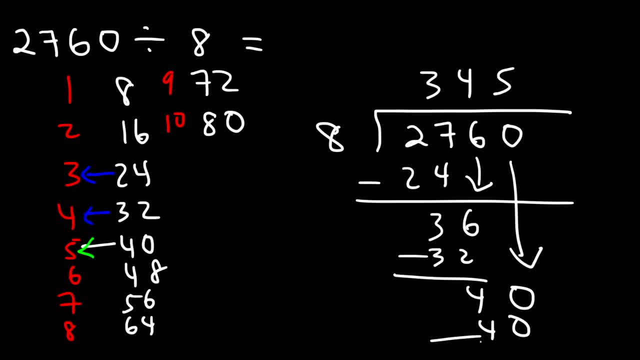 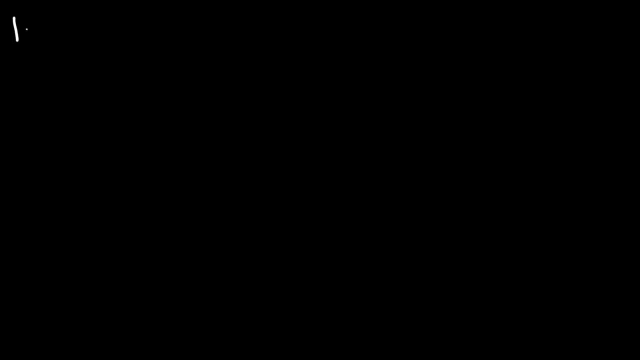 8 times 5 is 40, and the remainder is 0.. So at this point we could stop. So the answer is 345.. So 2760 divided by 8 is 345.. Now let's try a harder problem. 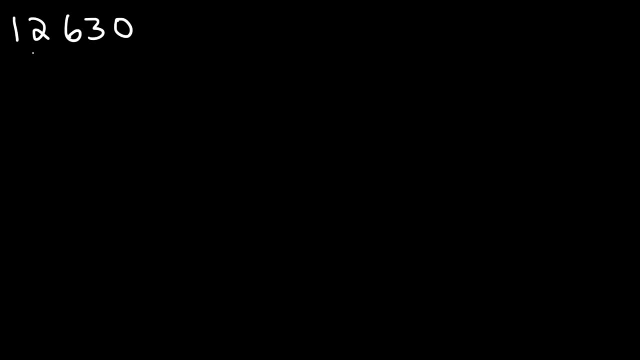 We're going to take an even bigger number- 12,630, and we're going to divide it by a 2-digit number, 15.. Go ahead and try this example. So we're going to put the numerator on the inside. 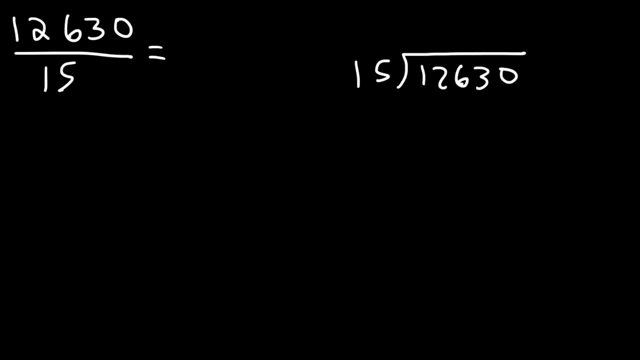 So let's write the multiples of 15 up to 10.. So we have 15, 30,, 45. Just keep adding 15 to each additional number. 60, 60 plus 15 is 75,, 75 plus 15 is 90, and then it's 105,, 120,, 135,, 150. So once you get all of that together, you're going to have a number of 15.. So once you get all of that together, you're going to have a number of 15.. And once you get up to 10, you can stop. 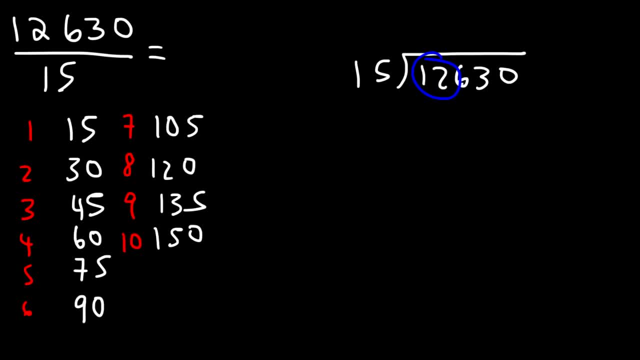 So let's begin. 15 does not go into 12, because 12 is less than 15.. 15 can go into 126.. Now, how many times? So what is the highest multiple of 15 just under 126?? This would be 120.. 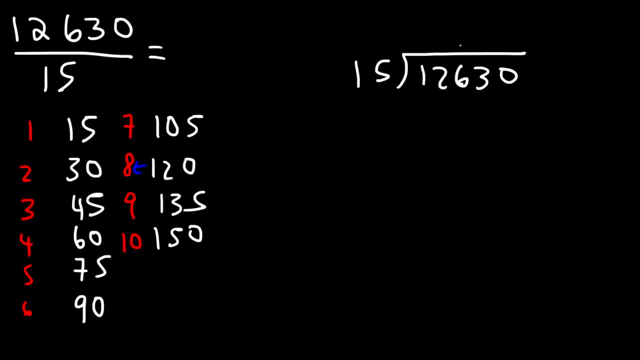 So thus 15 goes into 126. 126.. 8 times 15 times 8 is 120, and 126 minus 120 is 6.. Now let's bring down the 3.. Now let's move back to the chart. How many times does 15 go into 63?? 15 goes into 63 4 times. 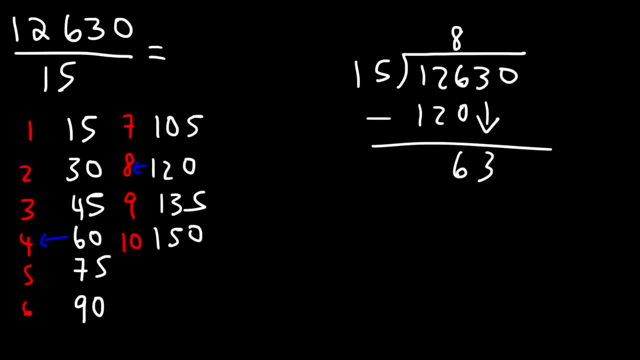 because 60 is the highest multiple of 15, just under 63. So let's put a 4 on top: 15 times 4 is 60.. 63 minus 60 is 3.. Now let's bring down the 0, and we can see that 15 goes into 30 exactly 2. 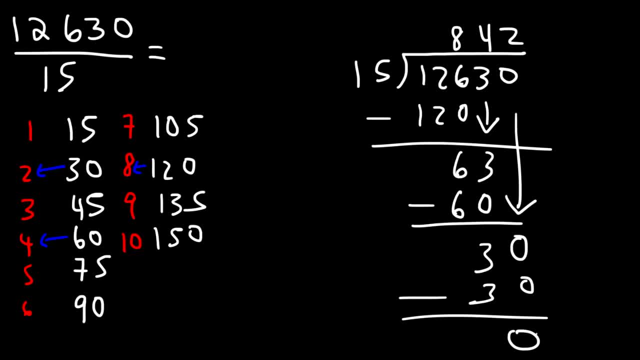 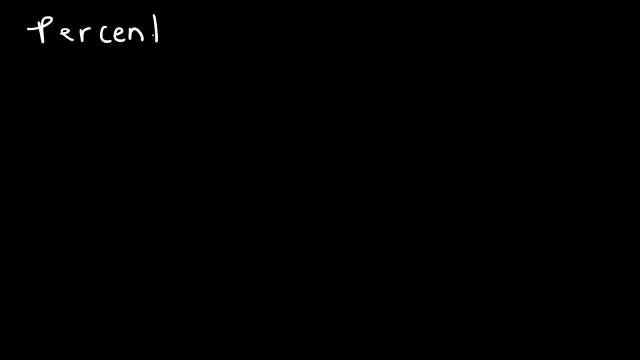 times 15, times 2 is 30, and the remainder is 0.. So the answer is 842.. So that's 12,630 divided by 15.. Now, the next skill we're going to talk about is percentages. So 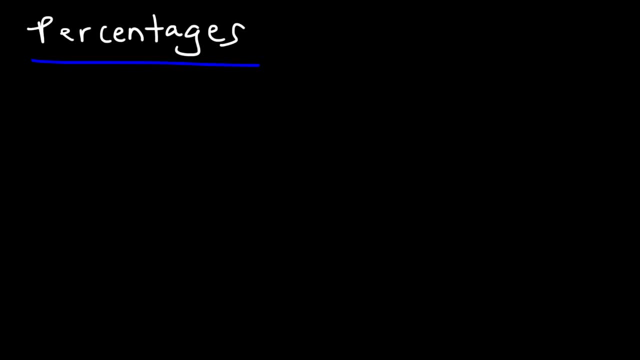 let's bring down the 0, and we can see that 15 goes into 30. exactly 2 times 15 times 2 is 30,. let's say you're at a restaurant and the waiter gives you an $80 bill. Now let's say you wish to. 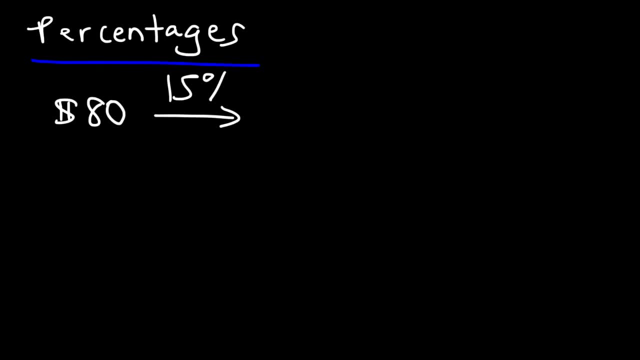 give the waiter a 15% tip and you're wondering: what is 15% of $80?? I don't have a calculator with me and my cell phone's battery is dead. So what is 15% of 80?? How can we figure this out? Well, 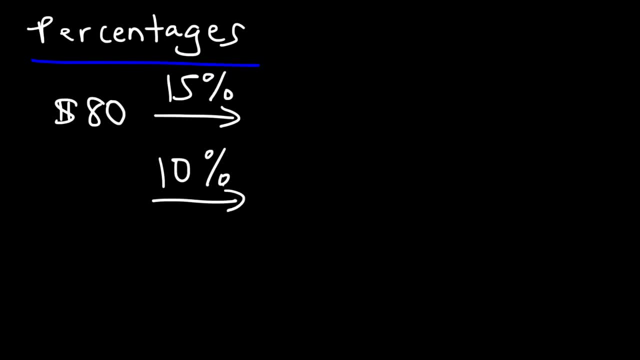 the best thing to do is find out what 10% of 80 is. To find out 10% of a number, all you need to do is take the decimal point and move it one unit to the left. So 10% of 80 is: 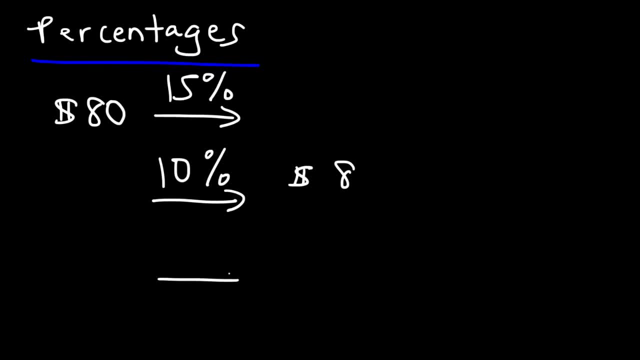 $8.. So if 10% is $8, what's 5%? 5% is half of 10%, So half of 8 is 4.. Now to find 15%, all we need to do is add 10% and 5%. So 15% of 80 is going to be 8 plus 4,. 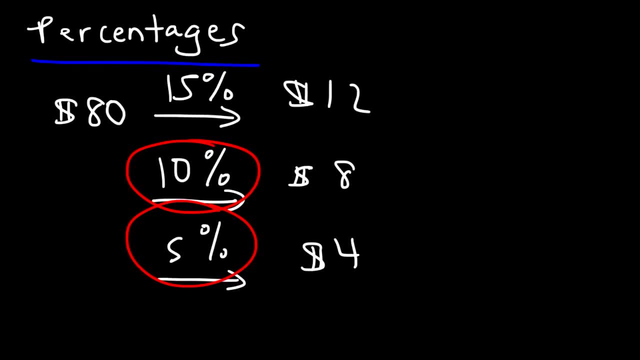 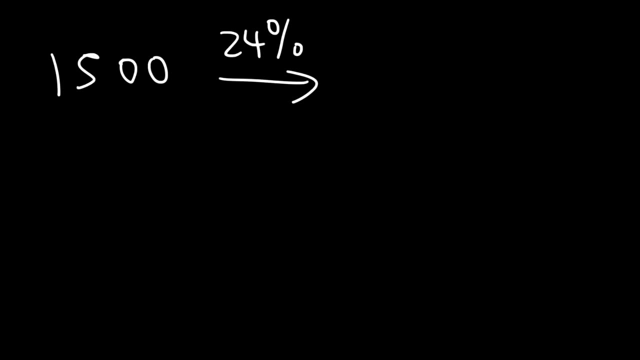 which is $12.. And so that's how you can do percentages in your head mentally. Let's try another example. So let's say, if we wish to find out what 24% of 1500 is, Feel free to try that problem. 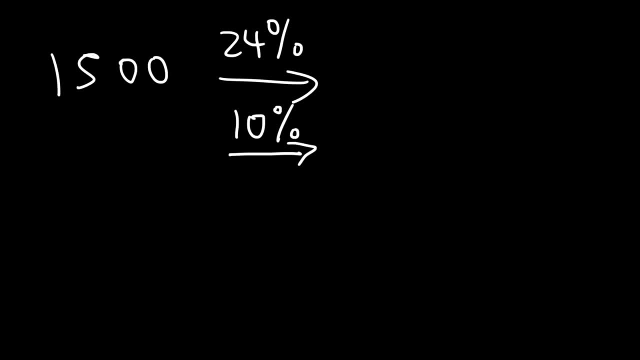 Let's begin with 10%. What is 10% of 1500?? So, once again, all we need to do is move the decimal point one unit to the left, So that will give us 150.. So if 10% of 1500 is 150, what's 20%? 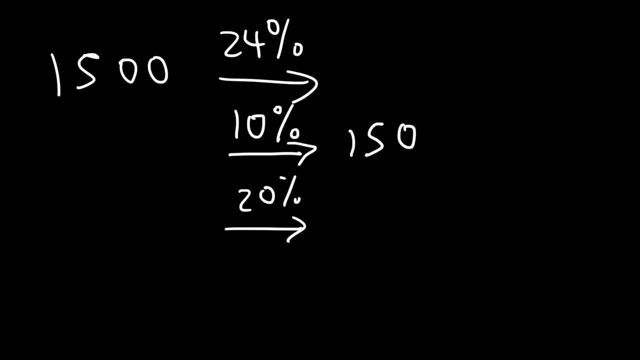 50 is 50.. 20% is simply twice 50. the amount of 10%, so what's twice the amount of 150? 150 times 2 is 300. now what is 1% of 1500? now, remember 10% was 150. all we have to do is move the. 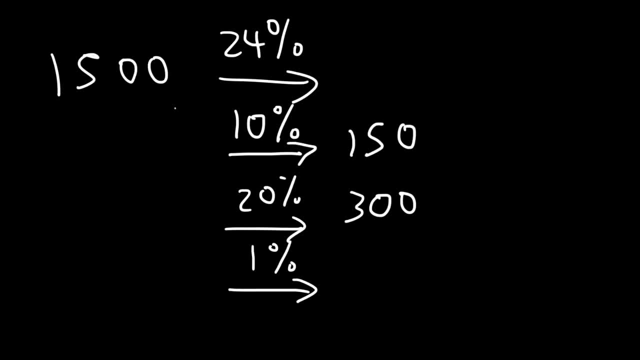 decimal point one unit to the left. to get 1% you need to move the decimal point two units to the left. so 1% of 1500 is 15. so what is 4%? 4% is 4 times the value of 1%. so basically we need to multiply 15 by 4. 15 times 4 is 60. so now 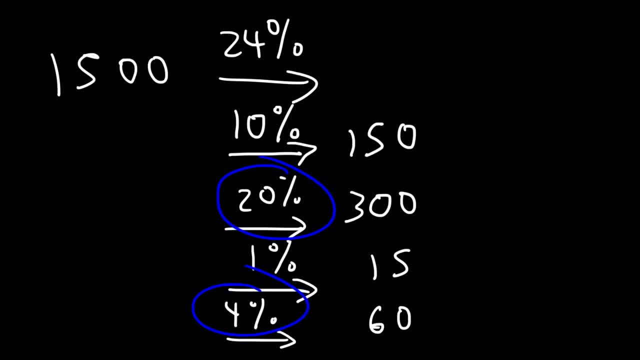 what we can do is add 20% plus 4% to get 24%. so we're gonna add 360, and so this will give us 60. so 360 is 24% of 1500. to confirm your answer, multiply 1500 by 0.24- 0.24.